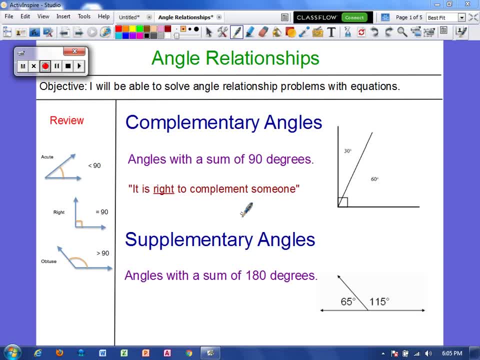 Hey everyone, Alright. today's video is over angle relationships, Your objective. I will be able to solve angle relationship problems with equations. So let's review: An acute angle is less than 90 degrees, A right angle is exactly 90 degrees And an obtuse angle is greater than 90 degrees. 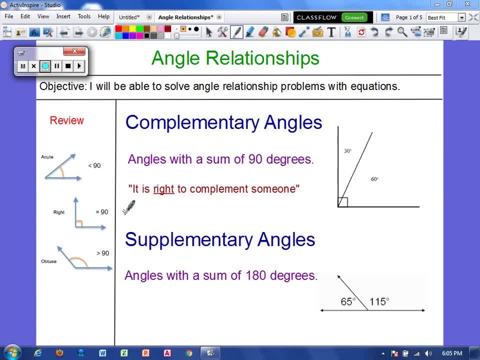 So let's talk about what complementary and supplementary angles are. Complementary angles are angles that have a sum of 90 degrees. So in this picture we see an angle of 30 and an angle of 60 degrees, And if we were to add those together, their sum would be 90.. 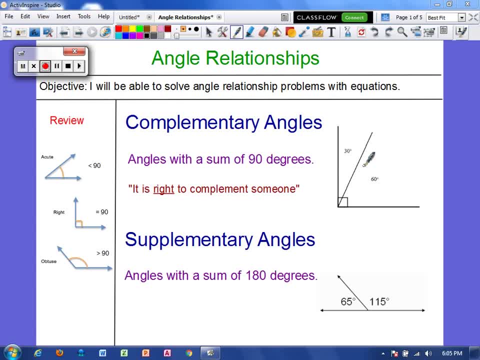 So these are complementary angles. So there are a couple of tricks to help you remember that. I like to say it is right to complement someone, And when we think of right we think of 90 degrees. or you can take the C in complementary and you can make a 9 out of it. 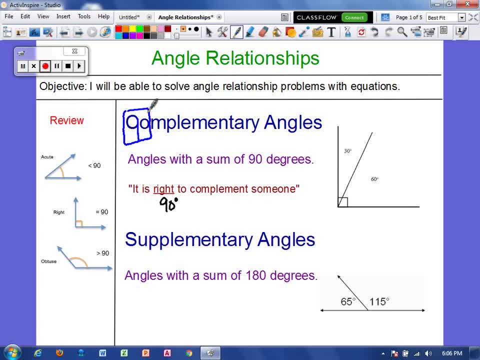 So then we see that 90 degrees Supplementary angles are angles that have a sum of 180 degrees. So in this picture, if we were to add 65 and 115, we would get 180.. And notice that supplementary angles form a straight line. 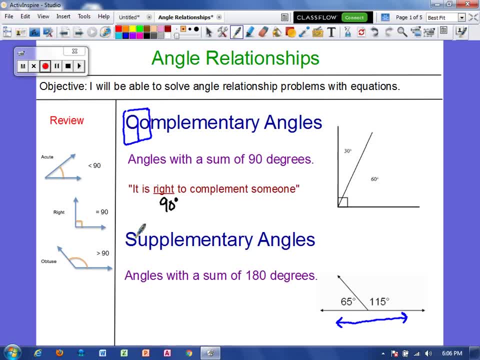 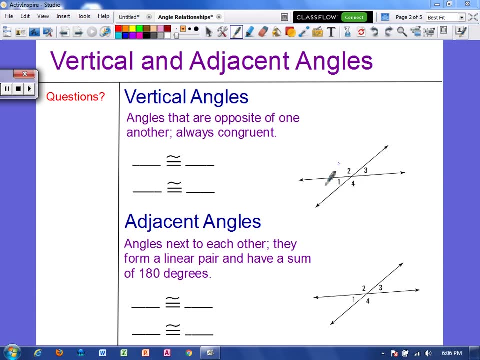 Now, as a trick for supplementary angles, you can take the S and you can make an 8 out of it. So you know, supplementary angles add up to 180 degrees. All right whenever we have two lines that are intersecting. 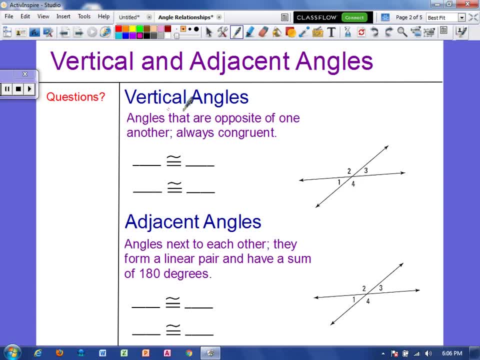 we have vertical and adjacent angles. Vertical angles are the angles that are opposite of one another And they're actually always congruent. So in this picture that means, if you can see the line of please zero, two, three, four, three, three, five, six, six, six, six, six, seven, eight, eight, eight hundred, and in these parts that means you have two lines intersecting, a vertical and adjacent angle. 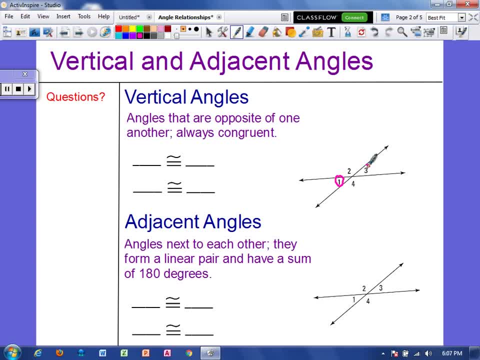 that angle 1 and angle 3 are vertical angles so they are congruent and, as you can see in the picture, the angles look like they would measure the same amount. so angle 1 and angle 3 would be congruent, and then angle 2 and angle 4. 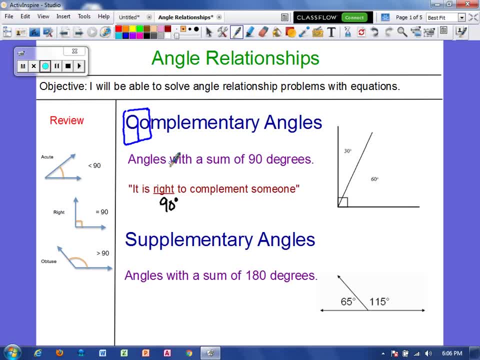 So then we see that 90 degrees Supplementary angles are angles that have a sum of 180 degrees. So in this picture, if we were to add 65 and 115, we would get 180.. And notice that supplementary angles form a straight line. 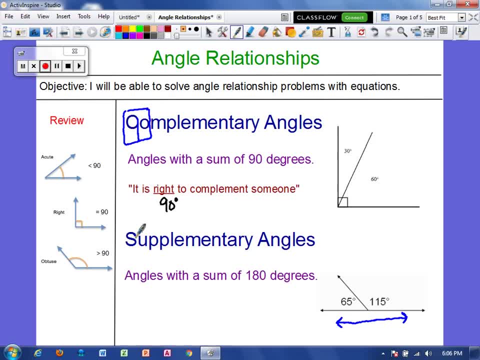 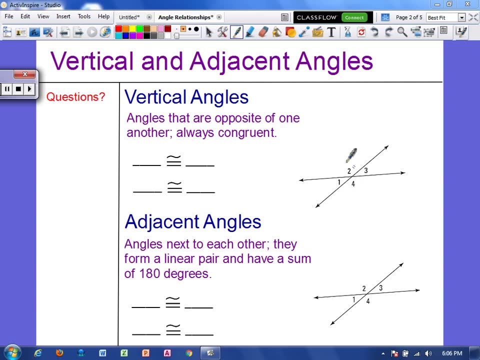 Now a trick for supplementary angles. you can take the S and you can make an 8 out of it. So you know, supplementary angles add up to 180 degrees. Whenever we have two lines or intersecting, we have vertical and adjacent angles. 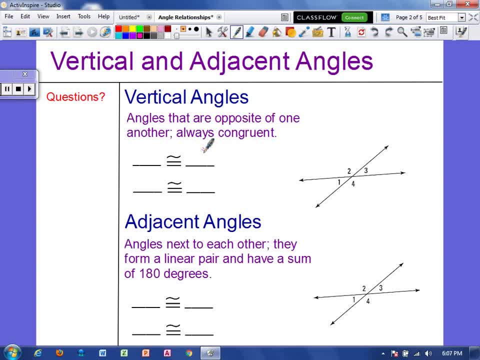 Vertical angles are the angles that are opposite of one another And they are actually always congruent. So in this picture that angle 1 and angle 3 are vertical angles, so they are congruent and, as you can see in the picture, the angles look like they would measure the same amount. 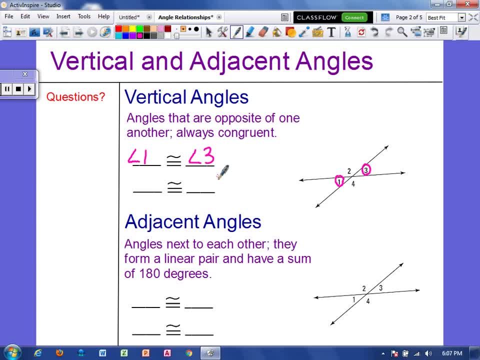 so angle 1 and angle 3 would be congruent, and then angle 2 and angle 4. those are vertical angles, so they would be congruent as well. now, adjacent angles are angles that are right next to each other and they form a linear pair, so as: 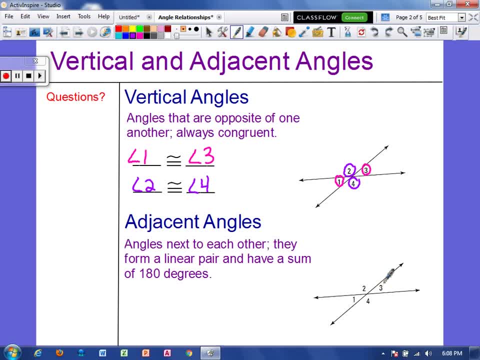 you can see here angle 2 and angle 3 are adjacent, angle 1 and angle 2, angle 1 and angle 4, angle 4 and angle 3. so any angles that are right next to each other, those are vertical angles. so you can see that they are congruent and they are. 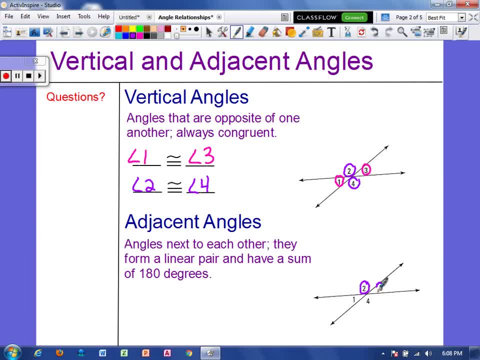 going to be adjacent and notice how they form a straight line. so they're going to add up to 180. so we could say that angle 2 and angle 3 are adjacent. and we could also say that angle 1 and angle 4 are adjacent, but you could say 1 and 2 are. 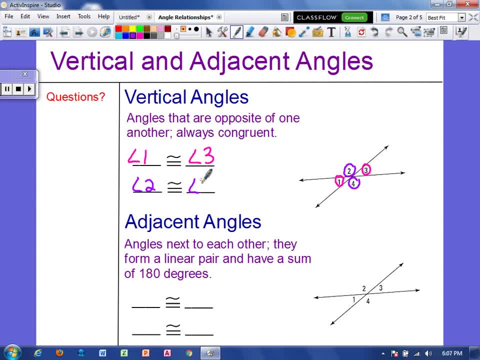 those are vertical angles, so they would be congruent as well. now, adjacent angles are angles that are right next to each other and they form a linear pair. so, as you can see here, angle 2 and angle 3 are adjacent, angle 1 and angle 2, angle 1 and. 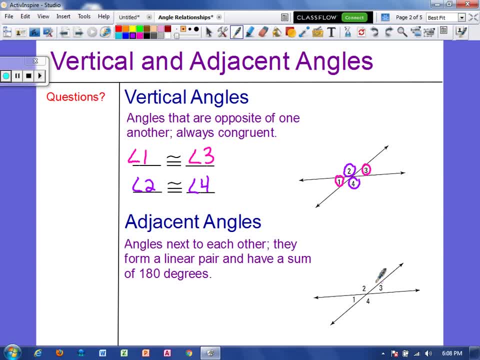 angle 4, angle 4 and angle 3, so any angles that are right next to each other, those are vertical angles. so now you can see here angle 1 and angle 3 are going to be adjacent and notice how they form a straight line. so they're going to 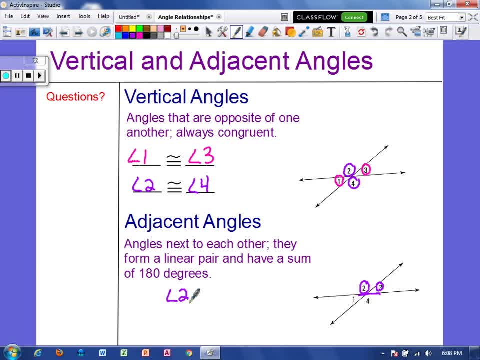 add up to 180, so we could say that angle 2 and angle 3 are adjacent. and we could also say that angle 1 and angle 4 are adjacent. but you could say 1 and 2 are adjacent, 3 and 4 are adjacent. it's up to you. but go ahead and write down two. 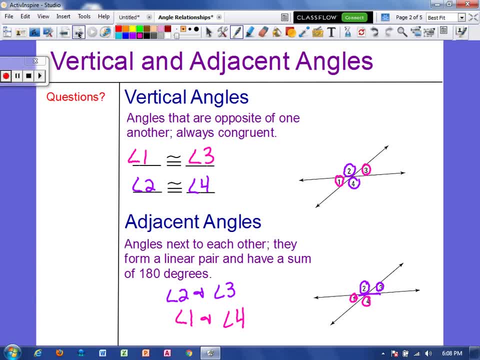 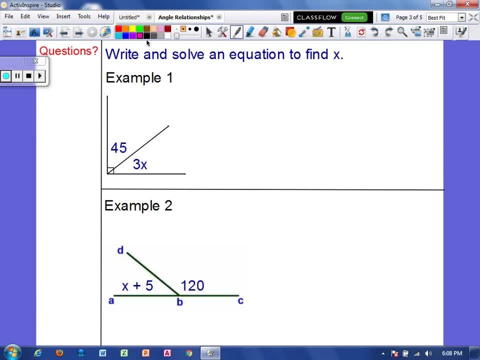 examples of adjacent angles. all right, let's solve some problems that involve angle relationships, and we're going to use equations to do that. so in example 1 we see an angle that measures 45 degrees, and we see an angle that whose measurement we don't actually know, if we're just represented with 3x, so we can. 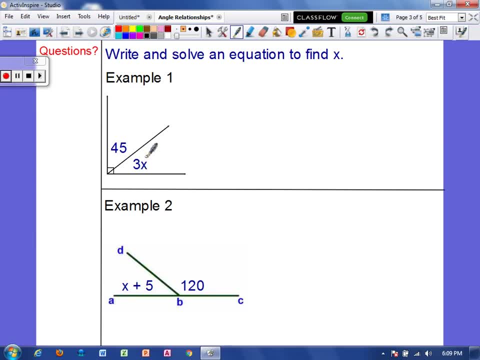 see that this is a 90 degree angle. so if I were to add these two angles together, we would have a 90 degree angle. so if I were to add these two angles, so if I were to add these two angles, so if I were to add these two angles, 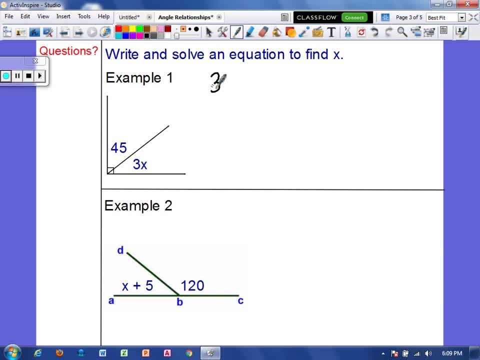 together it would equal 90 degrees. so that means 3x plus 45 would equal 90 degrees. now we just have a two-step equation, so I'm going to bring the equal sign down. I'm going to move the constant first. so we're going to subtract 45 on. 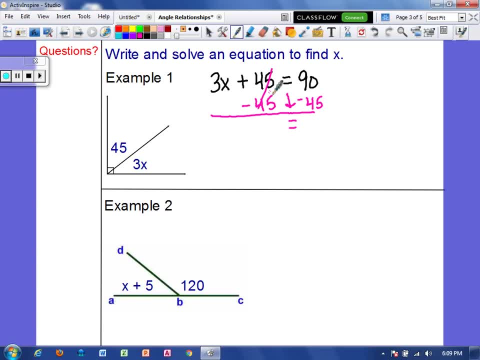 each side that cancels, we're left with 3x. 90 minus 45 is 45. the inverse of multiplying by 3 would be to divide by 3, so X would equal 15. so now I'm just going to check that. so 3 times 15 plus 45 should equal 90. 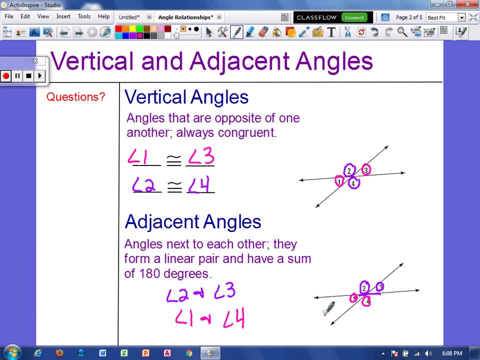 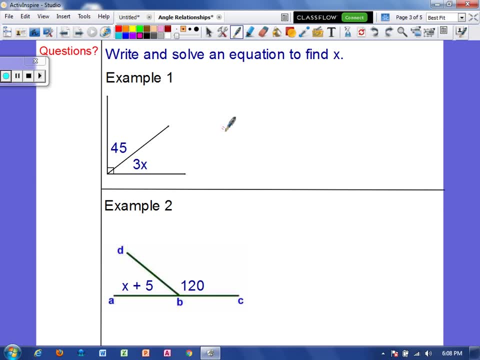 adjacent. 3 and 4 are adjacent. it's up to you, but go ahead and write down two examples of adjacent angles. all right, let's solve some problems that involve angle relationships, and we're going to use equations to do that. so in example 1 we see an angle that measures 45 degrees and we see an angle that whose. 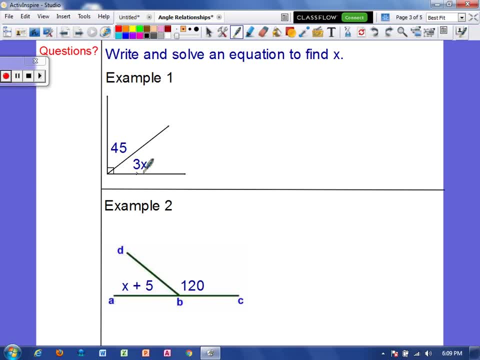 measurement. we don't actually know if we're just represented with 3x. so we can see that this is a 90 degree angle. so if I were to add these two angles together, we would have a 90 degree angle. so if I were to add these two angles, 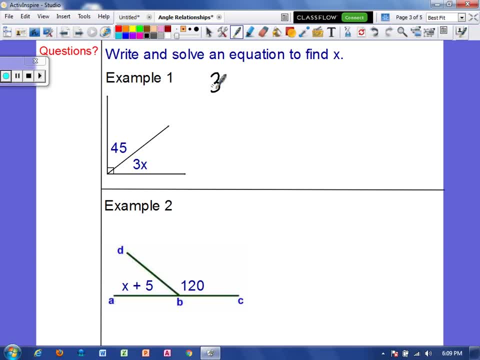 so if I were to add these two angles, so if I were to add these two angles together, it would equal 90 degrees. so that means 3x plus 45 would equal 90 degrees. now we just have a two-step equation, so I'm going to bring the equal. 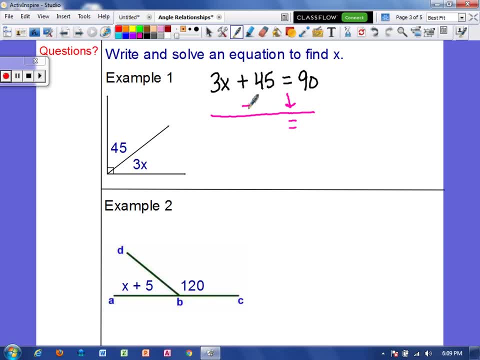 sign down. I'm going to move the constant first, so we're going to subtract 45 on each side. that cancels we're left with 3x. 90 minus 45 is 45. the inverse of multiplying by 3 would be to divide by 3, so X would equal. 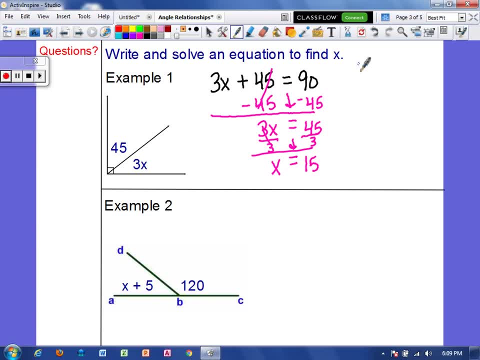 15. so now I'm just going to check that. so 3 times 15 plus 45 should equal 90. well, 3 times 15 is 45, and 45 plus 45 is 45. so 3 times 15 plus 45 should equal 90. 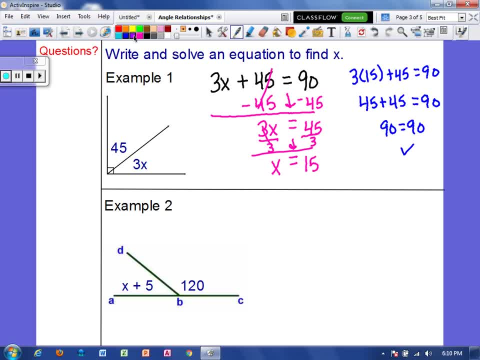 does equal 90. all right, in example 2 we have an angle that's represented by X plus 5 and we have an angle that's represented by 120 degrees. so I can see that these two angles are adjacent and they form a straight line. so that means 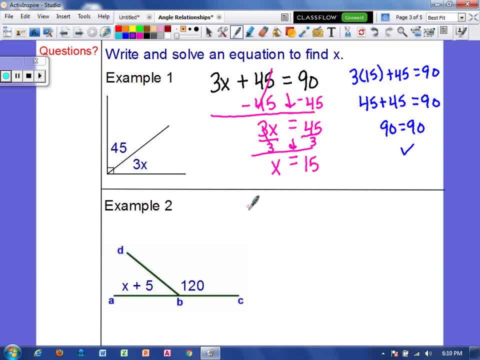 that they must equal 180 degrees. so if I were to add X plus 5 and 120 and then I divide by 5, it should equal 180 degrees. now here I have a 5 and a 120. I can actually combine those to make 125. that means X plus 125 equals 180. now I just 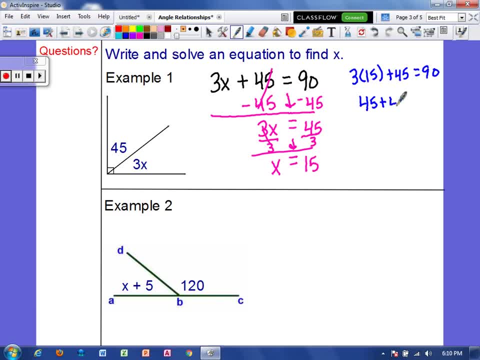 well, 3 times 15 is 45 and 45 plus 45 is 45. so we're going to divide by 3 and we're going to measure how much we're using to measure this consequence, the output. I need to be perfect, so I'm going to 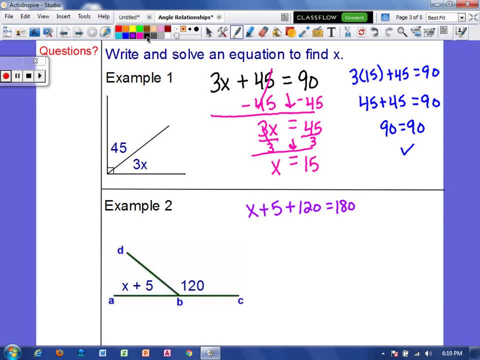 It should equal 180 degrees. Now here I have a 5 and a 120.. I can actually combine those to make 125.. That means x plus 125 equals 180.. Now I just have a one-step equation, So I'm going to subtract 125 from each side. 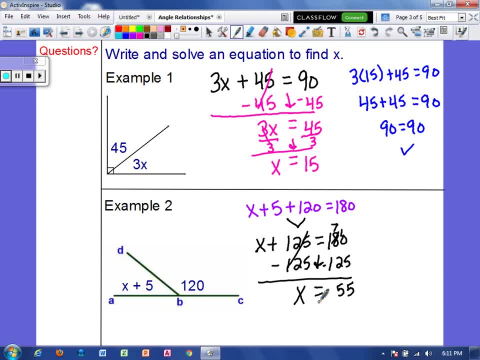 So x would equal 55. And if I were to check that that means 55 plus 5 plus 120 should equal 180.. Well, 55 plus 5 is 60, and 60 plus 120 would be 180.. 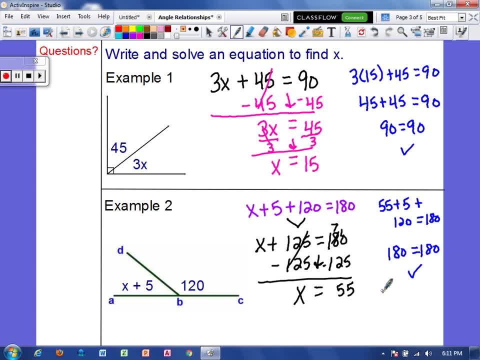 So we know that our answer is correct. Now, if the problem were to ask you what's the degree measurement for an angle, you would simply say: well, if x equals 15, 3 times 15 is 45. So this measures 45 degrees. 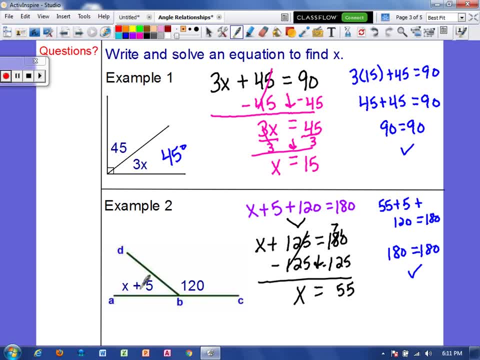 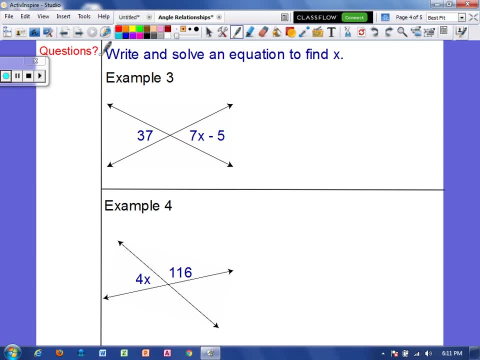 And for this angle we know x is 55. So 55 plus 5 is 60. So this angle would actually measure 60 degrees. All right, let's do some examples with two intersecting lines. So on example 3, we have some vertical angles. 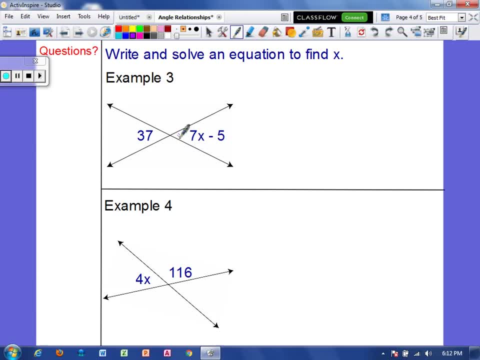 because they are opposite of 1.. We know that vertical angles are congruent, So that means that 37 must equal 7x minus 5.. So now we just have another two-step equation, So I'm going to add 5 to each side. 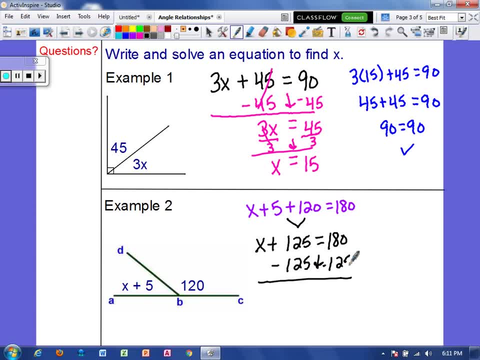 have a one-step equation, so I'm going to subtract 125 from each side, so X would equal 55, and if I were to check that that means 55 plus 5 plus 120 should equal 180. well, 55 plus 5 is 60 and 60 plus 120 would be 180, so we know. 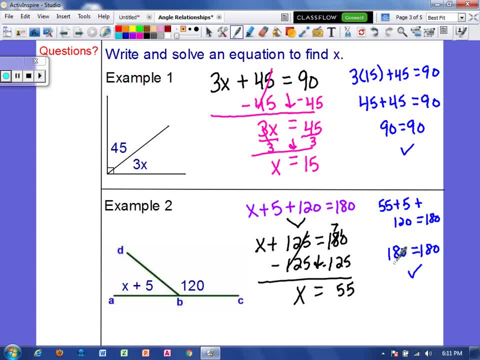 that our answer is correct. now, if the problem were to ask you what's the degree measurement for an angle, you would simply say: well, if X equals 15, 3 times 15 is 45, so this measures 45 degrees. and for this angle, we know X is 55, so 55 plus 5 is 60, so this angle would actually measure 60. 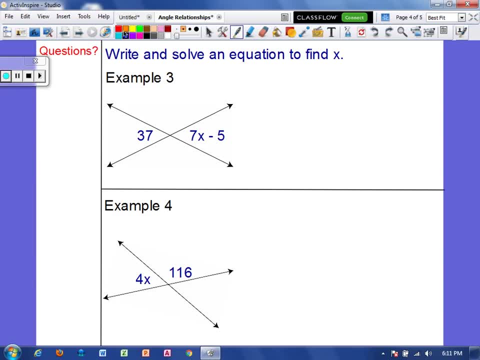 degrees. all right, let's do some examples with two intersecting lines. so on example 3, we have some vertical angles, because they are opposite of one another. we know that vertical angles are congruent, so that means that 37 must equal 7 X minus 5. so now we just have another two-step equation. so I'm going. 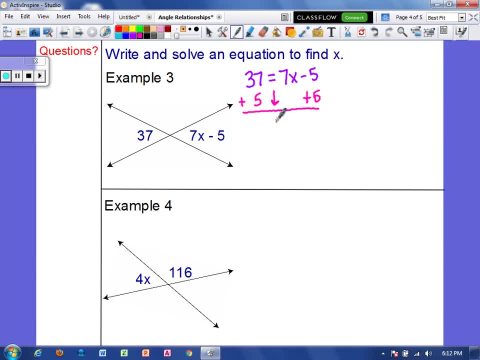 to add 5 to each side, 37 plus 5 is 42. you by 7 on each side, So x equals 6.. So now I'm going to check. So 7 times 6 minus 5 should equal 37.. 7 times 6 is 42.. And 42 minus 5 is 37.. And then obviously we know that this 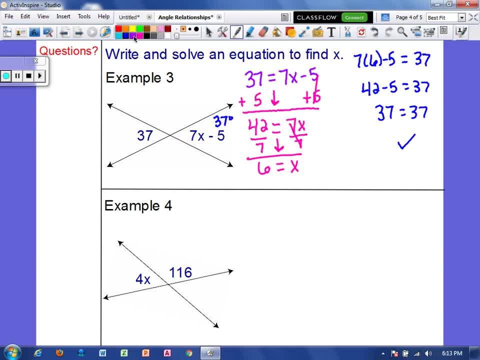 angle has to measure 37 degrees, since they are vertical. Alright, example 4.. We have adjacent angles. They are right next to each other and they form a triangle, So we have a straight line. So that means they have to add up to 180 degrees, So that means 4x. 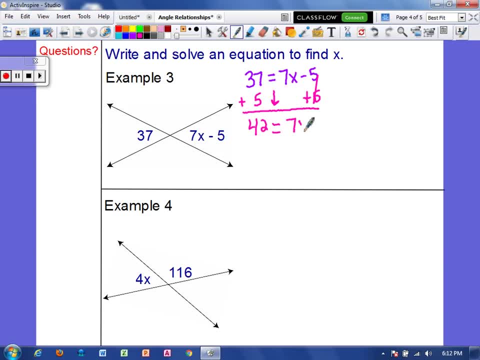 37 plus 5 is 42. 32.. I'm going to divide by 7 on each side, So x equals 6.. So now I'm going to check. So 7 times 6 minus 5 should equal 37.. 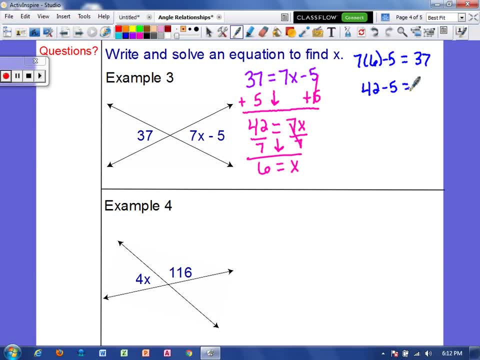 7 times 6 is 42.. 42. And 42 minus 5 is 37.. And then, obviously, we know that this angle has to measure 37 degrees, since they are vertical. All right, example 4, we have adjacent angles. 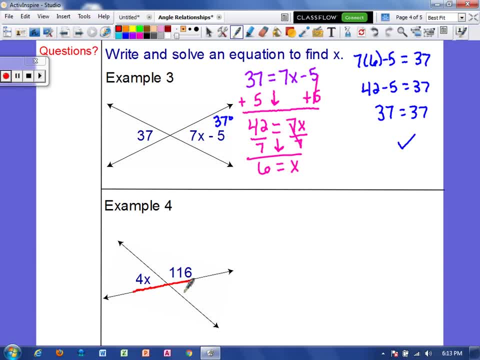 They are right next to each other and they form a straight line. So that means they have to add up to 180 degrees. So that means 4x plus 116. equals 180 degrees. So I'm going to subtract 116 from each side. 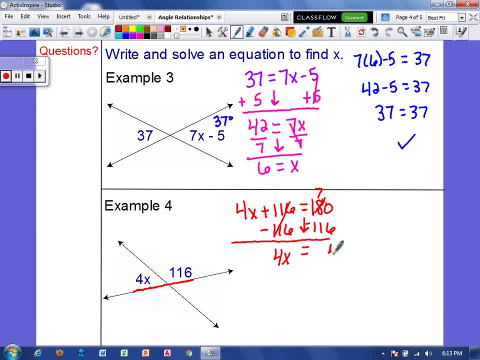 I'm going to have to borrow: 10 minus 6 is 4.. 7 minus 1 is 6. And 1 minus 1 is 0. So now we're going to divide by 4 on each side, And I'm going to come over here to the side to work that out. 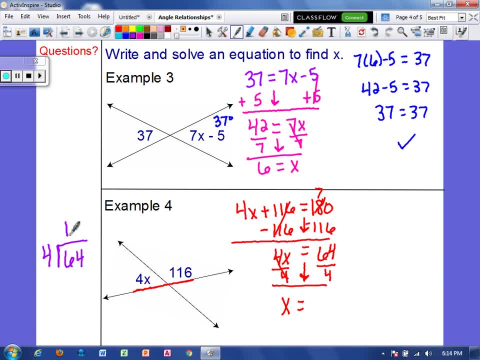 So top dog goes in the house, 4 goes into 6 one time with 2 left over, And 4 goes into 24 six times So x would equal 16.. So let's check that. So that means 4 times 16 plus 116 should equal 180.. 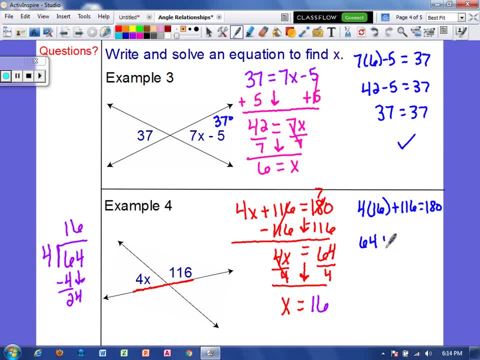 Well, we know, 4 times 16 is 64. And if I were to actually work out, 116 plus 64.. 6 plus 4 is 10.. 2 plus 6 is 8.. We do get 180.. So we know that our answer is good.